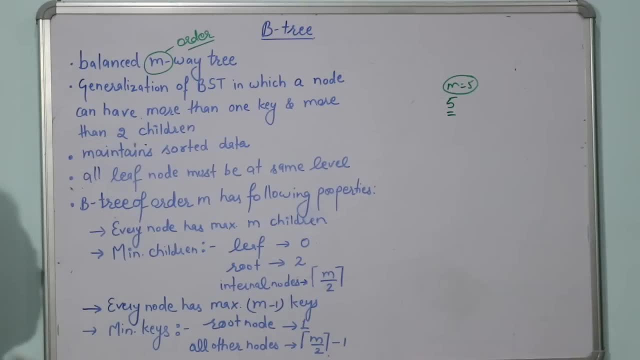 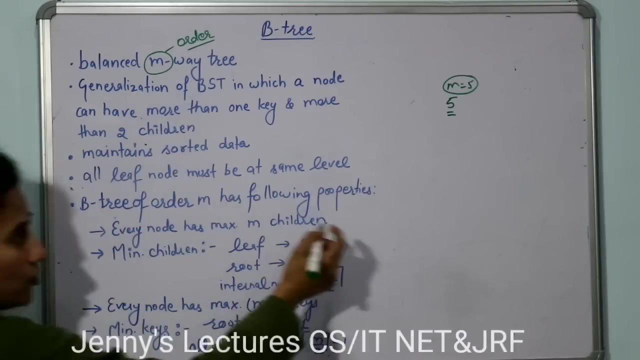 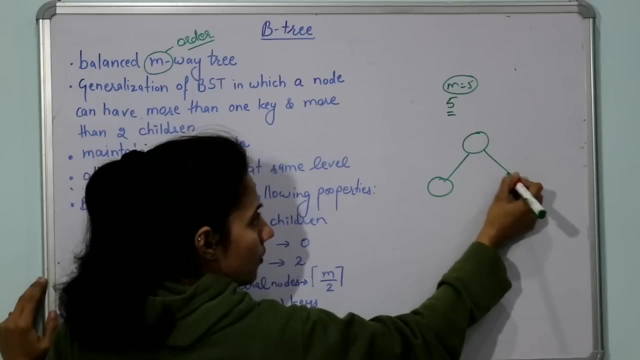 That tree would be 5-way tree. Okay, it is also known, as you can say it is generalization of BST, BST, BST is what That is. binary search tree: Okay, I hope everybody know what is binary search tree In which a node can have more than one key and more than two children. See in case of binary tree. or you can say binary search tree. binary means what? Two, So every node can have at most two children. That is case of binary. See at most two children. I am not saying exactly. 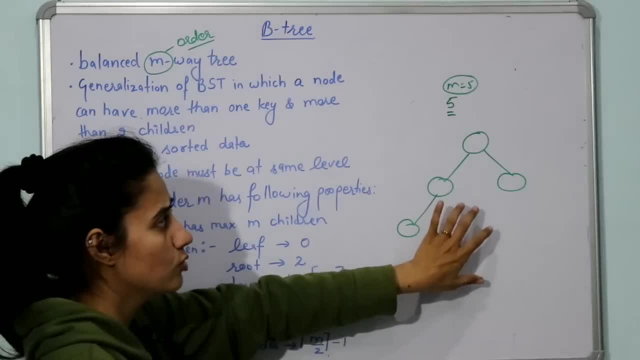 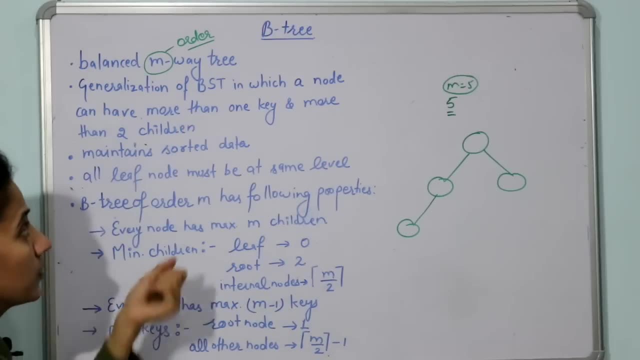 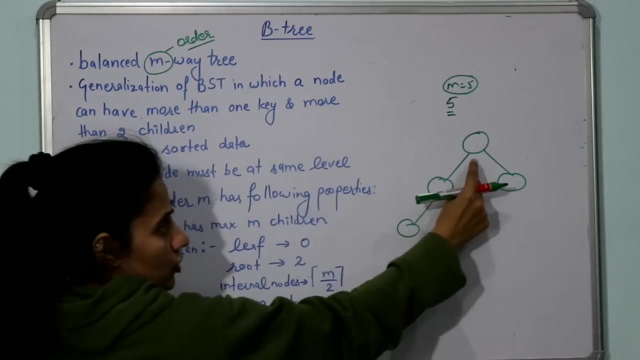 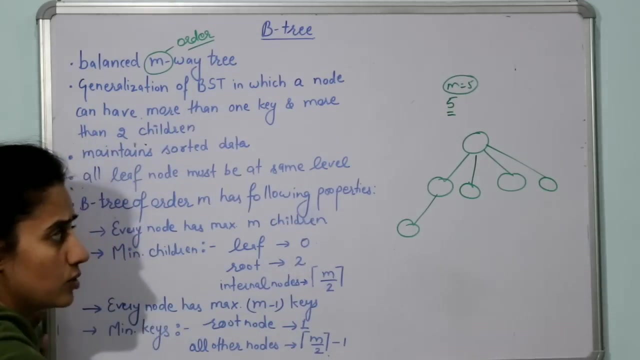 Two children. One children can be, zero can be, but at most two children will be. That is the. you know meaning of binary, Binary tree or binary search tree. you can say: But in case of B-tree, these are not binary tree. We can say because children can be more than two children: One, two, three, four, five, six. How many children can be It depends on the value of M. We will discuss it with the help of an example. 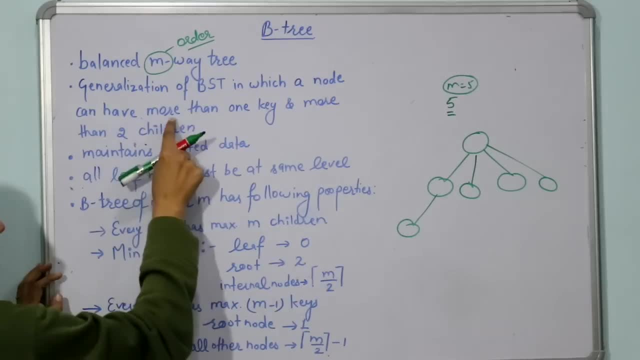 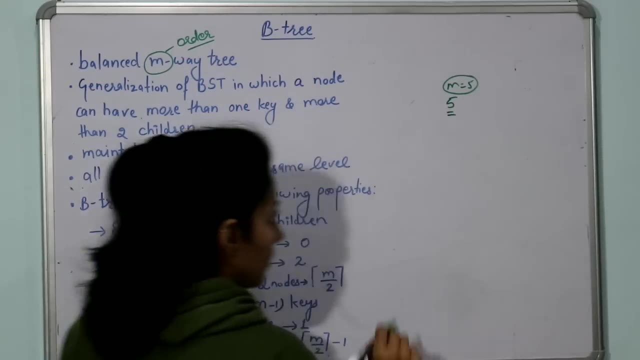 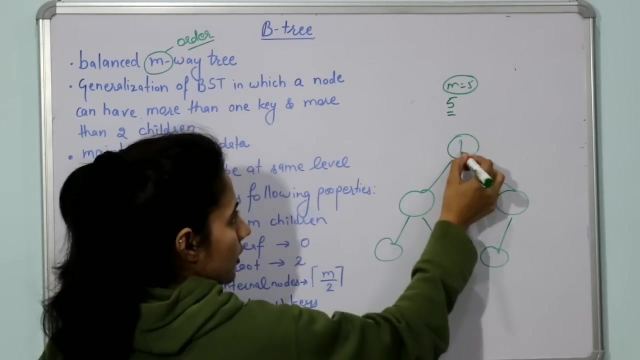 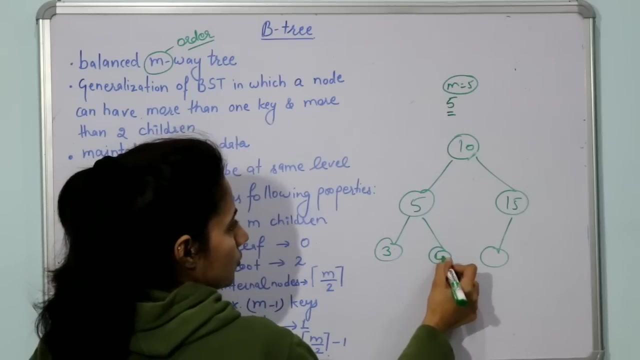 One more thing is: every node can have more than one key. See key means what? Let us take one example of binary search tree. Suppose this is binary search tree. Here we have 10. Here we have 5.. Here we have 15.. Here we have 3. Here we have 6. And here we have 11. Suppose 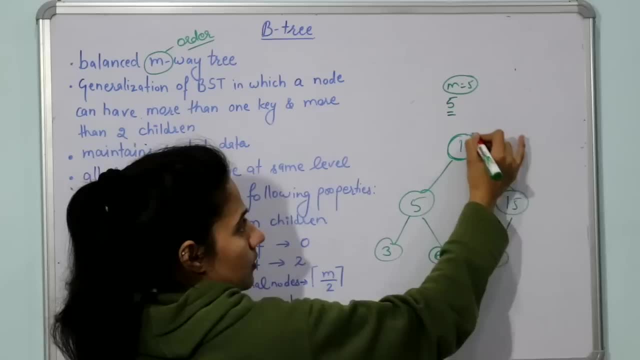 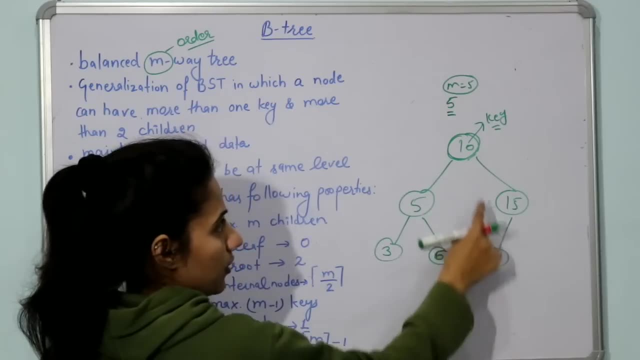 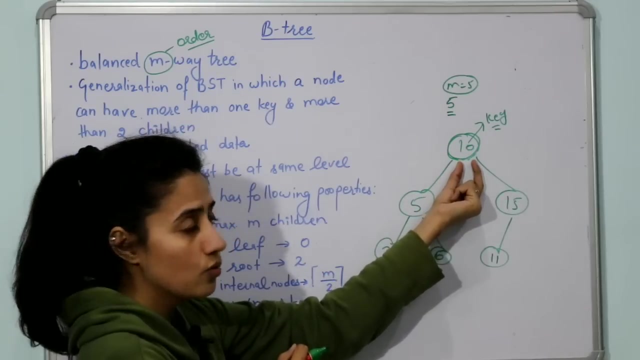 Okay, So this is known as node And the value is known as key value, Or you can say key: One node is there, One node, one node, node and node. Every node is having how many keys? Only one key. See, here the key value is 10.. That is, key is 10.. So every node can have only one key, But in case of B-tree, a node can have more than one key. 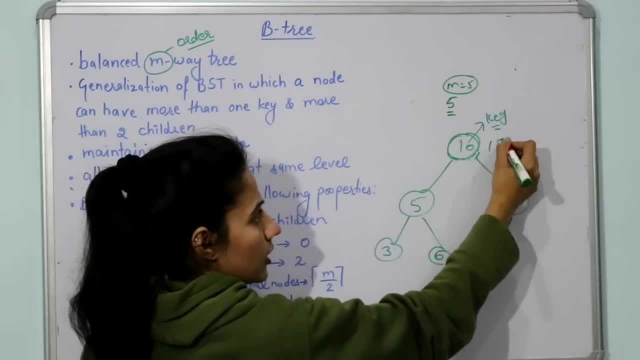 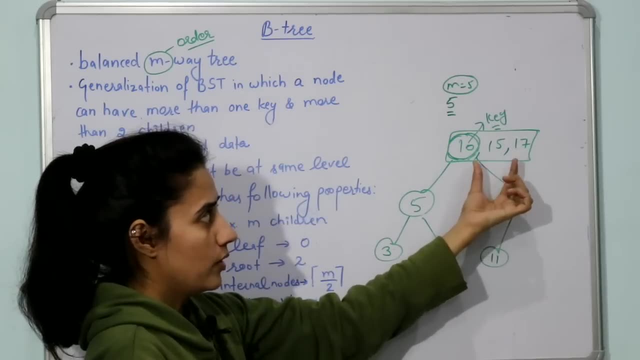 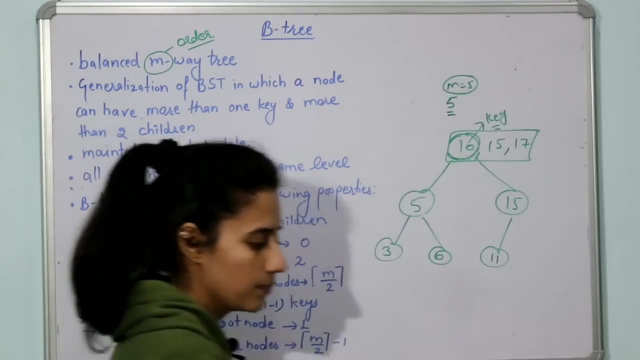 Here. if you create B-tree here, you can write 15 along with 10.. You can write 17 too, And that would So every node can have more than one key, And how many keys would be there in this node It would depend on the value of M. Okay. 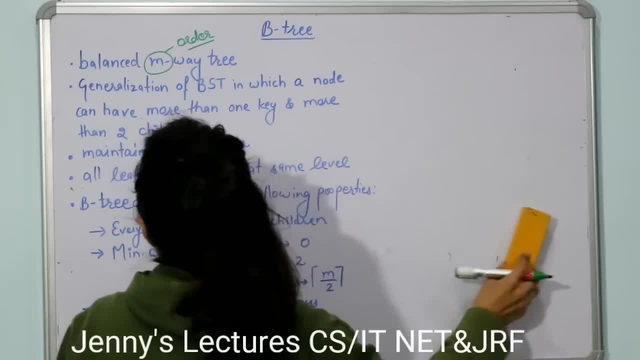 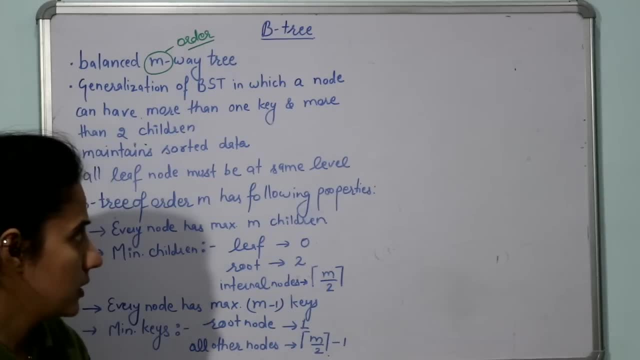 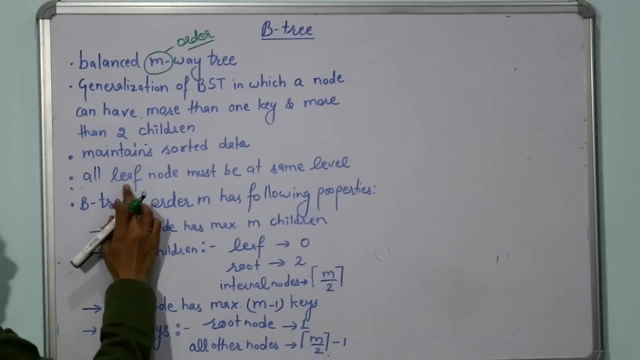 Now the next point is it always maintains the data in, you know, sorted data, Or you can say in ascending form. We will discuss it with the help of an example. Next is all the leaf node must be At the same level. in B-tree, Same level means C. 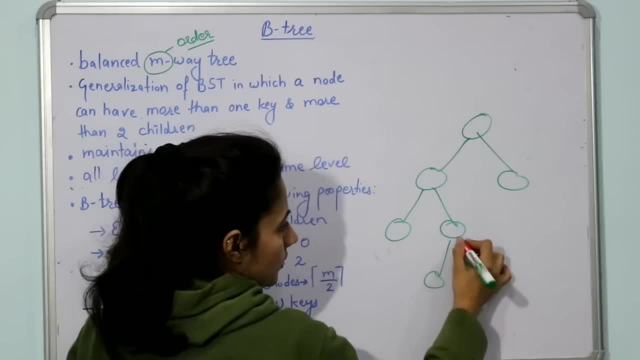 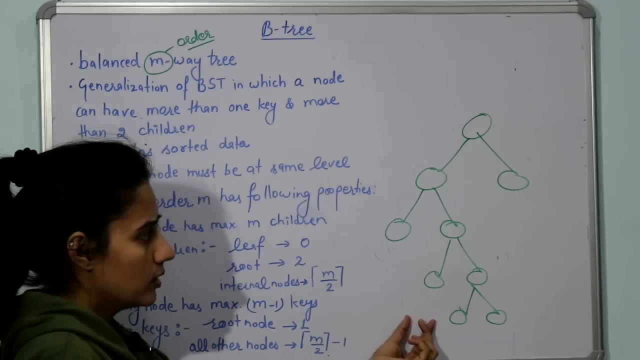 We saw a tree, This, this, Suppose, this one, this one, this one And this one. Okay, Obviously, this is also a binary tree And you can say binary search tree. If you write, you can give values here. 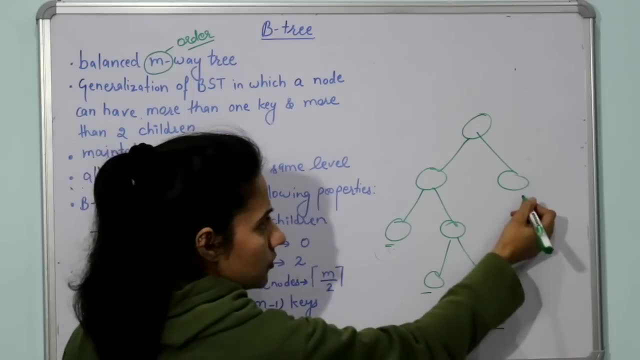 This one is leaf node. This one is leaf node. This one is leaf. This one is leaf, This one is leaf. But every leaf node is at different, different level. Suppose, here you take 0th, You take 1 level. 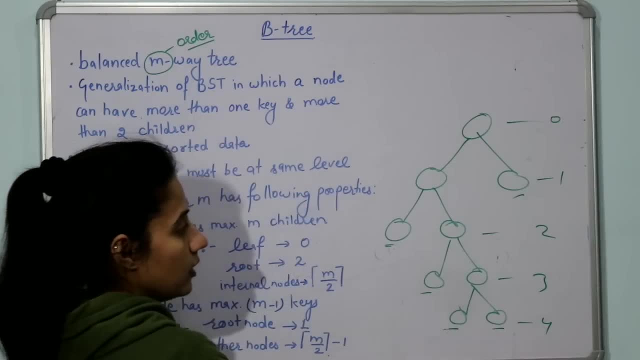 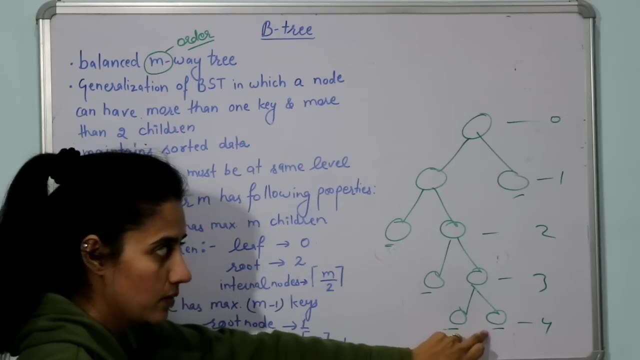 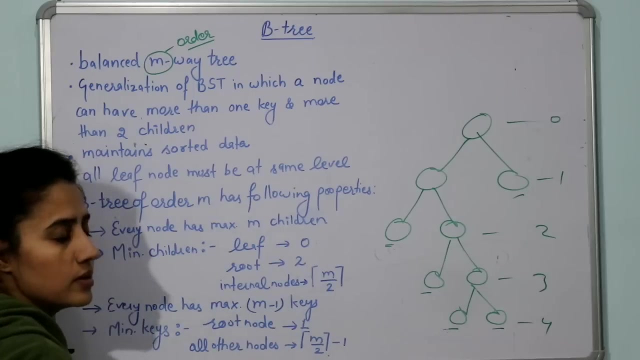 You take 0th, You take 0th. this one is third, this one is fourth. okay, so every node is having at a different level, but in B tree every, sorry every- leaf node is at different level. it is possible in bindwell trees, but in case of B tree every leaf node must be at the same level. wo same level. pe hi honge. 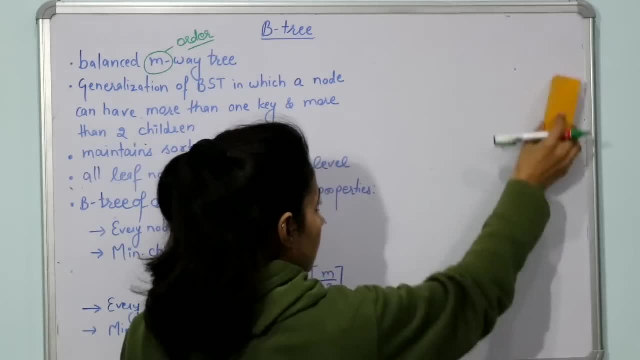 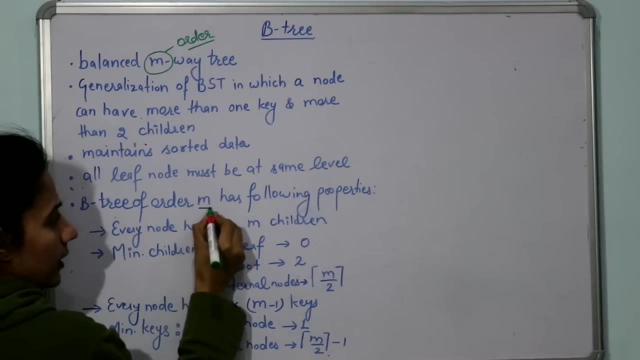 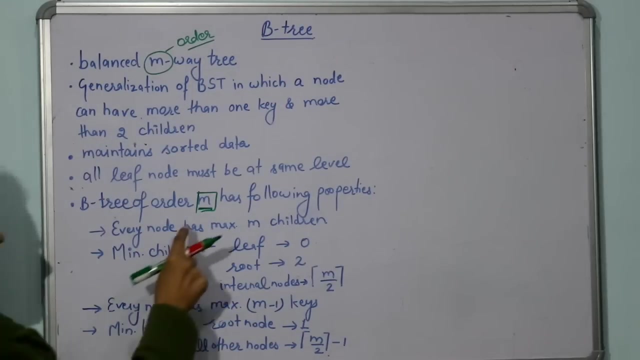 example lehenge. in that case, then it would be clear to you: okay, now if we have order M, then a B tree of order M has the following properties: us properties honge agar uska order M hai. M means wo three, four, five, kuch bhi ho sakta. it would be given in example: see order M hai. in that case, 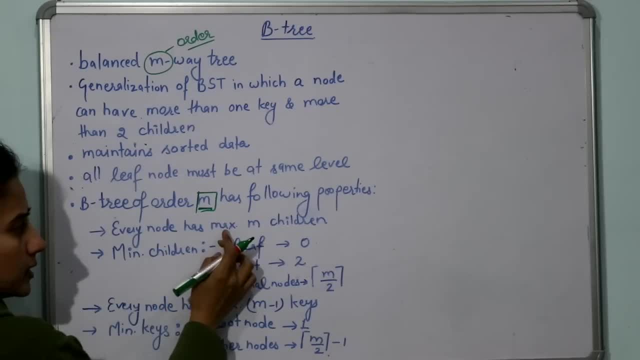 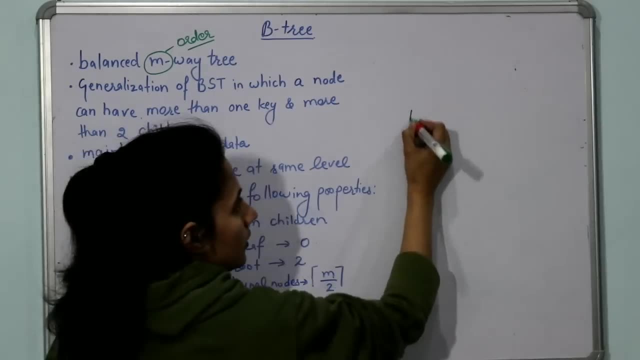 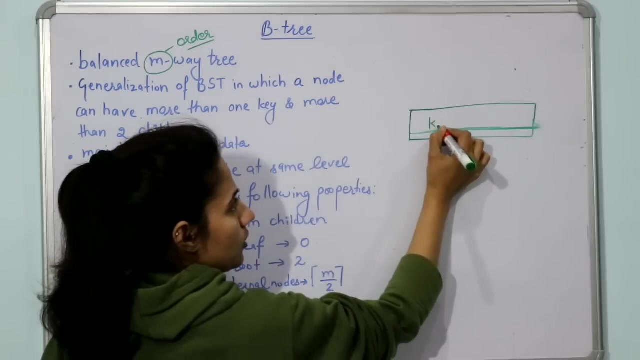 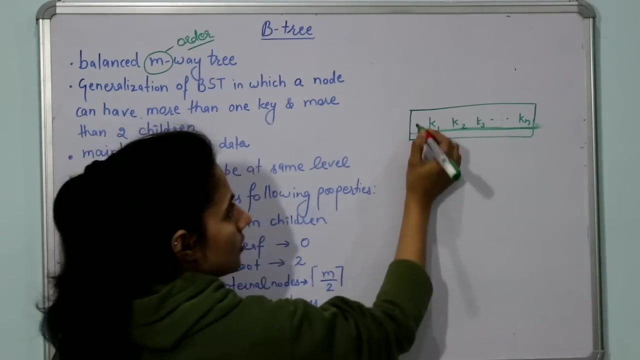 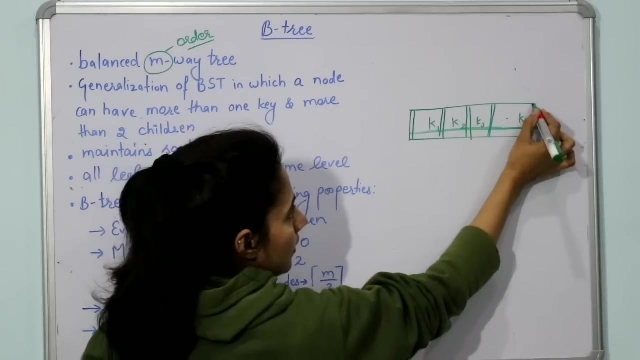 every node has m maximum m children, at most m children. okay, every node is ka data data structure, B tree ka kuch aisa hoga node ka see like this: every node can have more than one key, like key one, key two, key three and up to k suppose key n. okay, and it would also be having some pointer so you can say links. 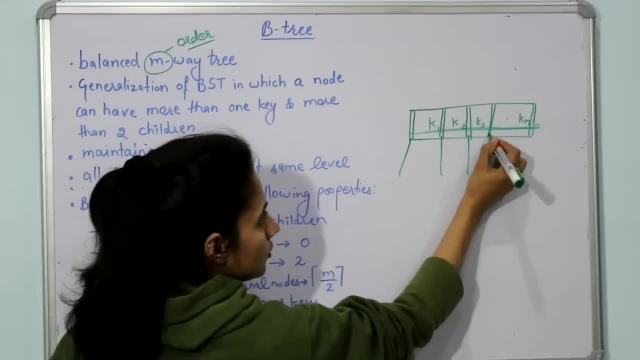 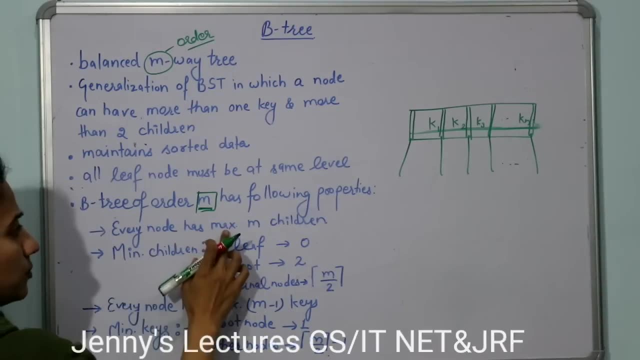 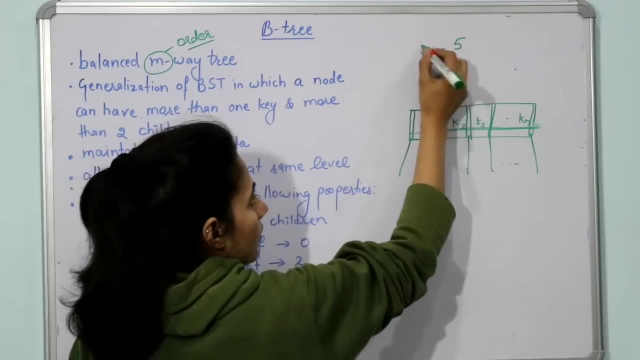 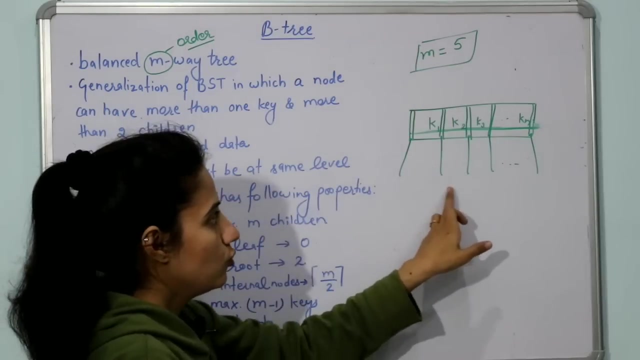 and these links would be to the. you know children. you can say these are children of this node. okay, so every node has maximum m children. suppose a B tree of order five is given. suppose M key value is five. so every node can have maximum how many children? only five children: one, two, three, four, five. 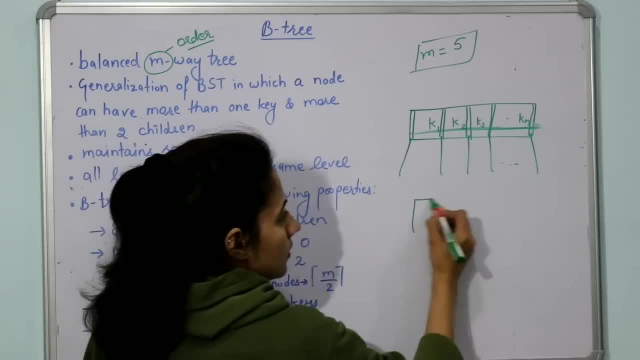 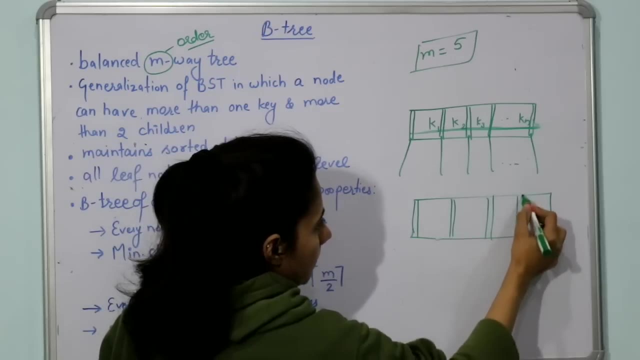 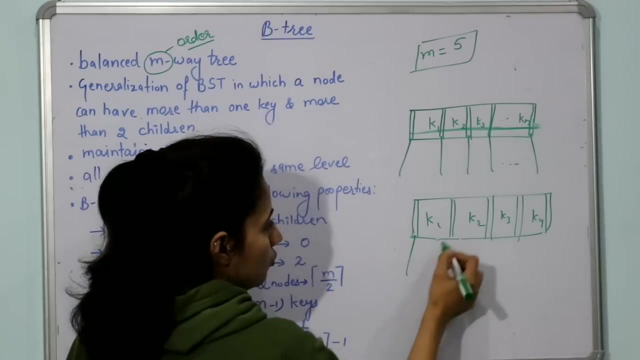 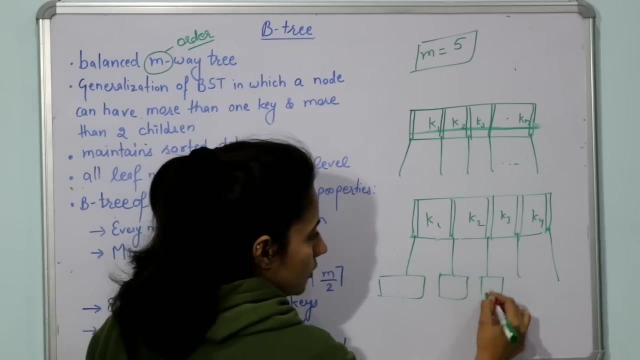 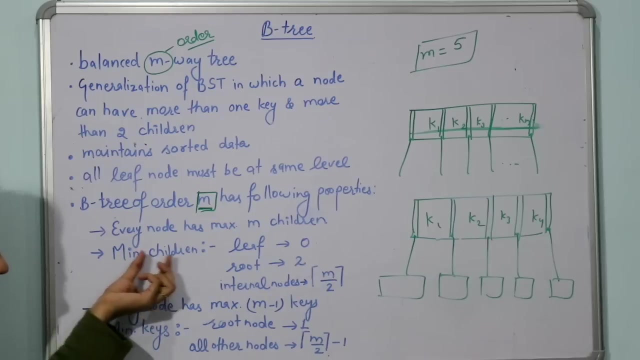 links could be there. okay, see K one, k two. these are in information. uh, sorry, key values. one, two, three, four and five. these are children, or you can see surprise children, okay, and minimum children. it may move, suck there. maximum children: m Hっていう'll check my channel below and you also curious to see. okay, this is definitely useful and you also know A-SAT words for step and crossتى. that's why I am sharing this here. okay, so these are some viral from this lesson. I will share it with you. I hope you like this Warning. see you on those who like this. that's all very anything. you know thoseسdeh comments and I'll share my things. that's, it's cool, what so it? this point exactly means all do a lot. correct are different questions based income view readers: K 1, K, 2, K filled, k1, two & 2. these are information sorry key values. one, two, three, 4 and So on. 1, 2, 3, 4 and 5- these are children, but you can say sub breeze, at most 5 children, okay, & minimum children. how many kids? 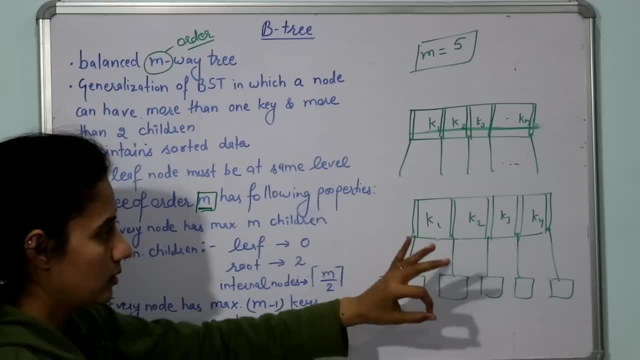 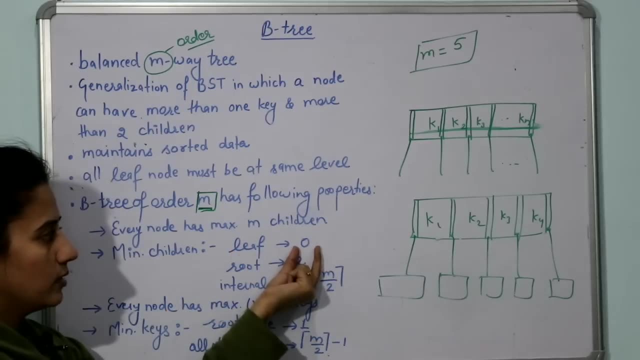 M for every node. for root leaf and all the internal nodes Minimum children will be. obviously there will be no child of leaf node. that is means zero children. For root node, minimum children would be two. it's only for that root node, okay. 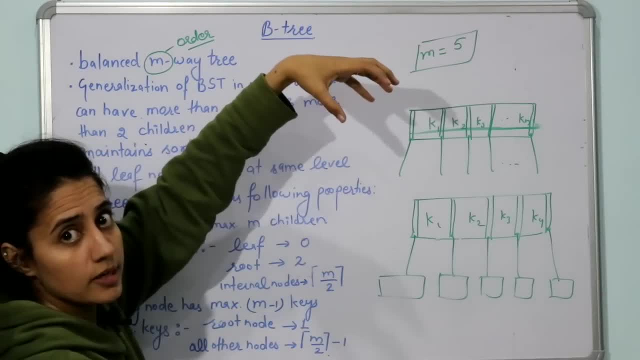 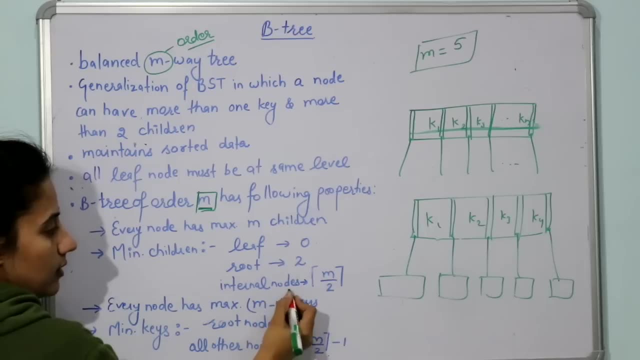 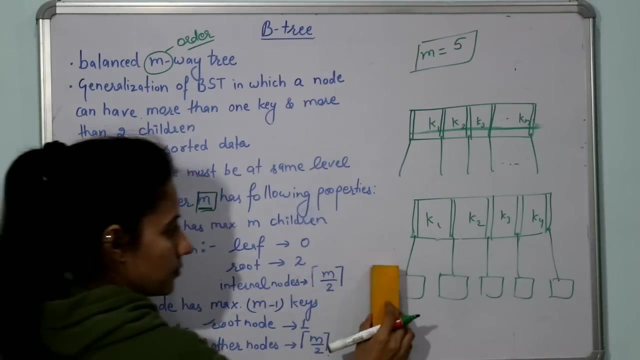 Root node will be in starting and below that are leaf nodes. so all the nodes in between that are known as internal nodes, And all the internal node would have minimum how many childrens M by 2, and this one is ceiling, see ceiling. I hope everybody know. suppose here we take. M is equal to 5, then 5 by 2 ceiling. 5 by 2 means 2.5, if we take ceiling in that case, what would be the answer? that is 3.. 2.5.. It is real number value in point. so the integer above it, just above it, that would. 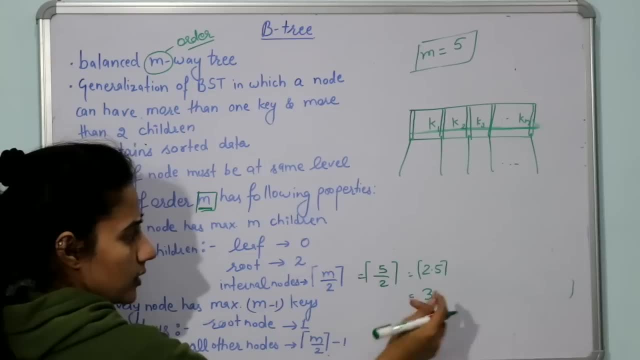 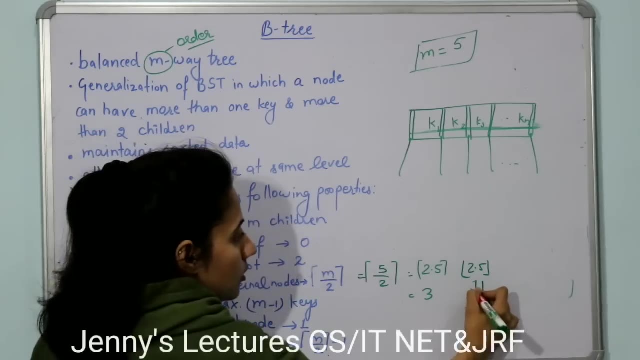 be 3.. Ceiling means we will take above 3, if it is floor. in that case, if we have to take floor value of 2.5, floor means below value- then you would have taken that 2,, okay ceiling. 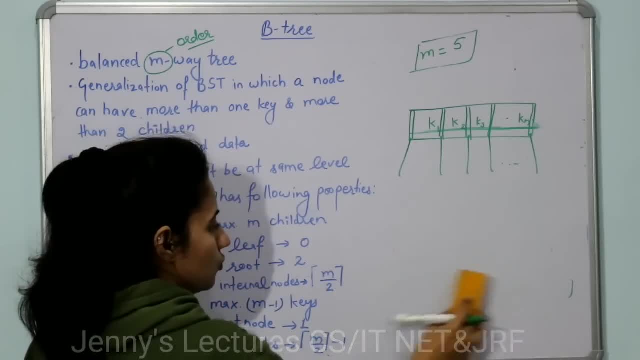 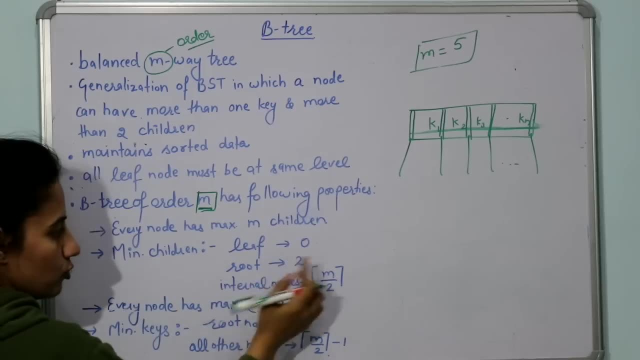 means 3.. 5 by 2, ceiling of 2.5 will be 3.. Children will be maximum M, children, Minimum children. leaf will be nothing for root. minimum 2 and all the internal node will have M by 2 and its ceiling. 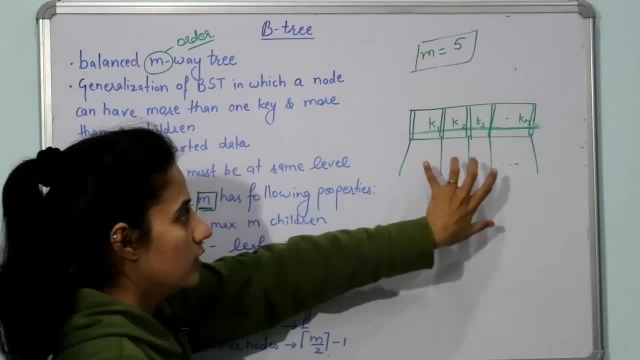 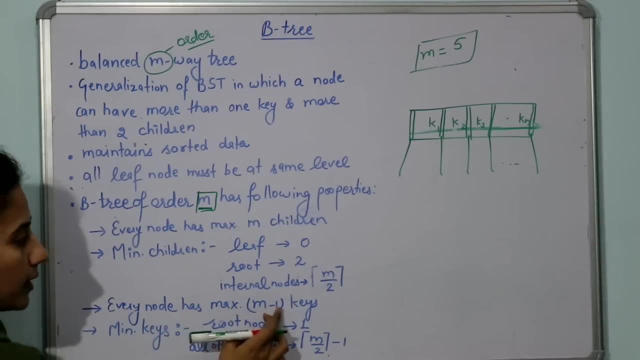 Now next is how many keys would be there. this keys will be of children or not. now, how many keys will be? that would be: every node has maximum M minus 1 keys means how many children will be there. one key will be less than them maximum. if there are M children, then M minus. 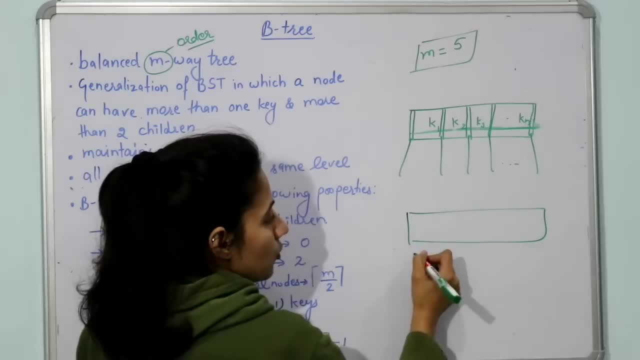 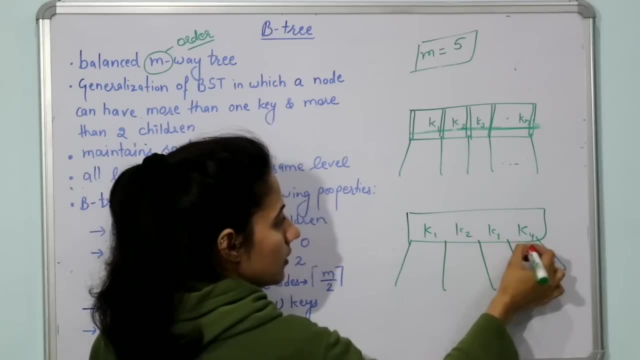 1 key. Suppose here how many. we had 1 key, 5, 1, 2,, 3,, 4,, 5, so how many keys will be there? K1,, K2,, K3 and K4.. Maximum key would be- these are links: K1, K2, K3, K4, for every node. Now, minimum keys would be: for root node, minimum key would be 1, see it's for root node minimum key. how many can be 1.? 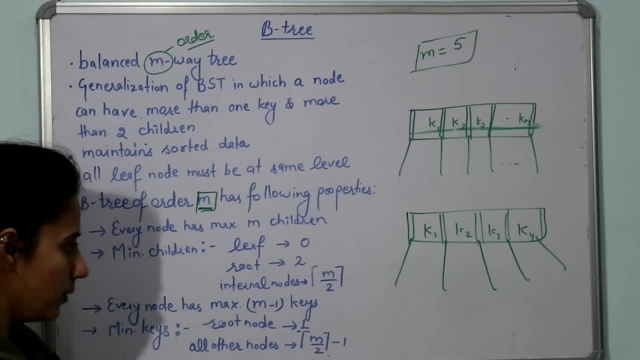 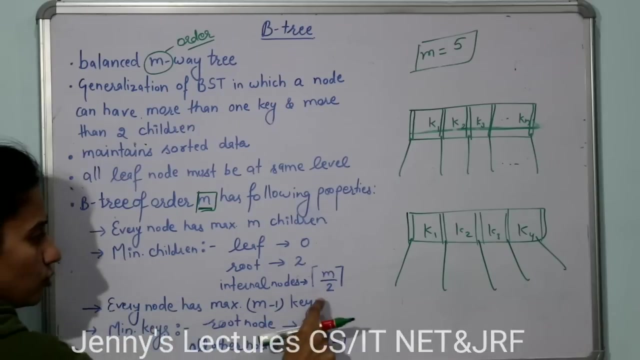 Except root node, for all the nodes, all other nodes would have minimum keys M by 2, ceiling minus 1.. You don't have to get confused in this: minimum children would be M by 2 ceiling and minimum keys would be M by 2 ceiling minus 1, here also what will be your 1 minus maximum keys: 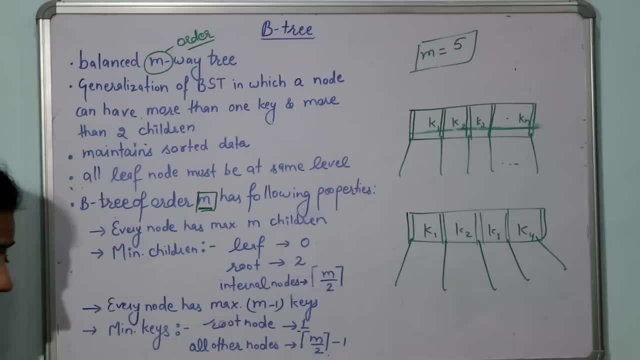 M minus 1, and maximum children would be M by 2 ceiling minus 1.. Minimum keys would be M by 2 ceiling minus 1.. Minimum keys would be sum minus 1,, 2,, 5,, 6,, 7,, 7,, 8.. 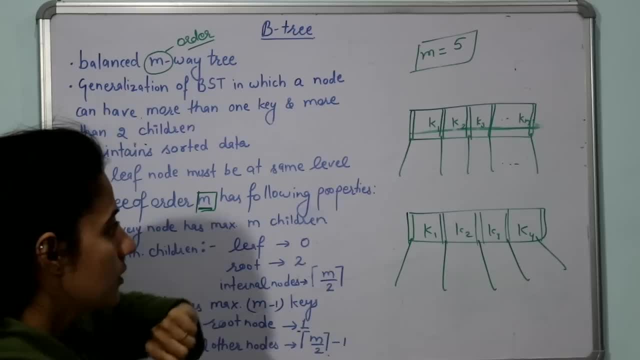 But this is for minimum: 1, 1,, 2,, 3,, 4,, 5,, 6,, 7,, 8 or minimum key to be given. It can be blamed on M M. Okay, One more thing about B-tree. 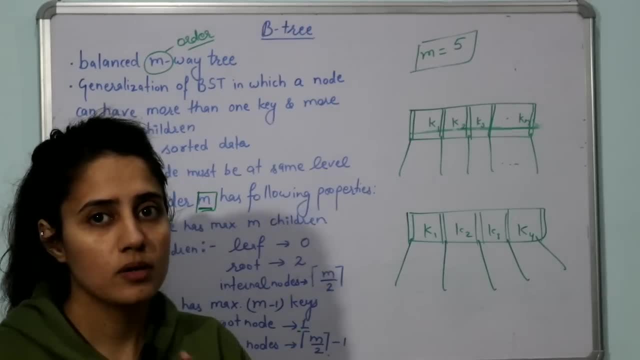 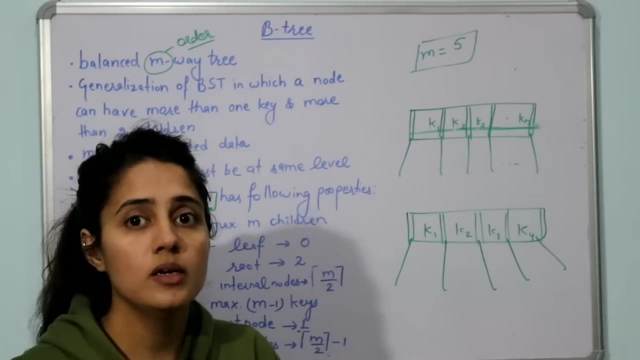 See, in this case, in these type of trees, the insertion would be always in the leaf node. Okay, If you want to insert some value, that value would be inserted in the leaf node only. You won't insert it in the root. it would always be inserted in the leaf node. 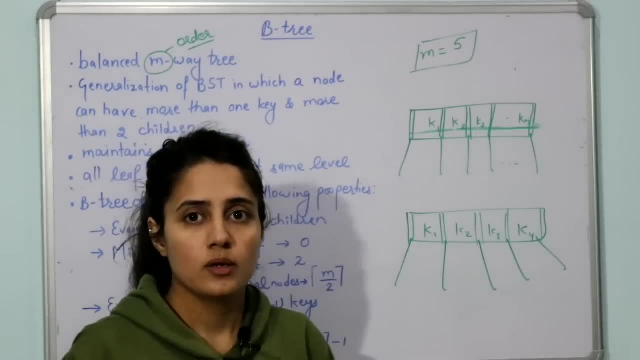 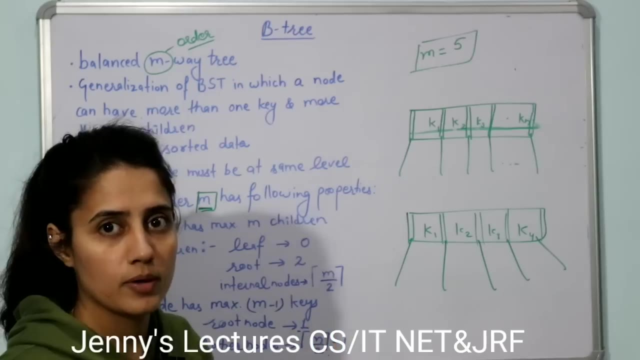 Okay, So in next turn we will talk about 0 to M. Okay, So next turn I will explain this OK video. i will take one example and i will discuss how to create btree using these properties. till then, bye, bye, take care.